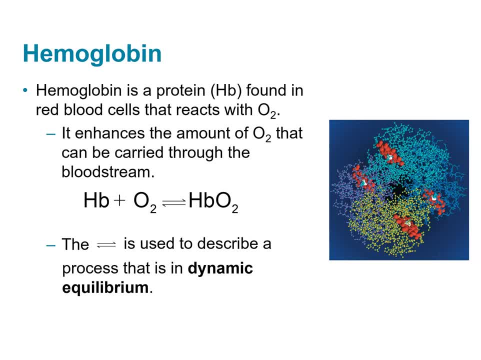 and have a general feel for, since it's our main transport mechanism, Our oxygen in our blood, And it's also happens to be a really good example of dynamic equilibrium and how equilibrium can change based on all of the components that are participating in a reaction. 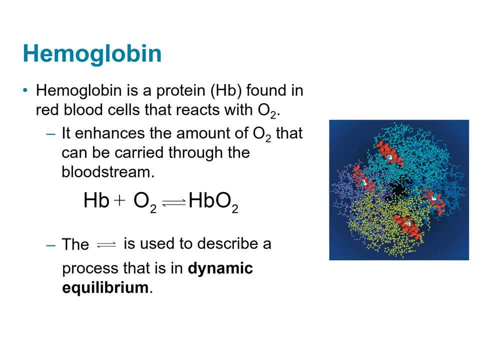 So hemoglobin, which is subtitled HB, is found in our red blood cells and it binds oxygen gas. And when it binds oxygen gas, we can look at this reaction And say: hemoglobin as a reactant binds oxygen gas as a reactant, and when hemoglobin is bound to oxygen, that is our product. 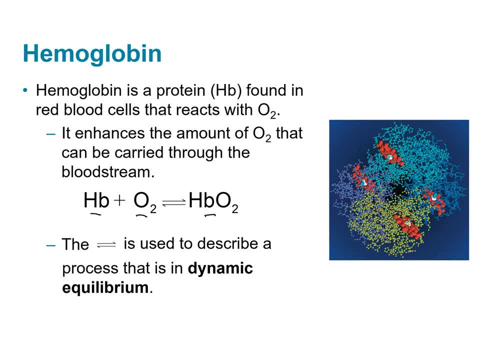 And you'll notice right away that we're using this double-sided arrow to describe something which we call dynamic equilibrium And the double-sided arrow, whereas we've typically seen reactions, progress with a forward arrow. oh, that's a terrible arrow. let me 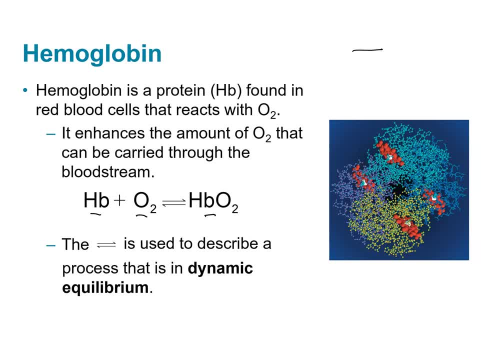 Let me try that again. Drawing on tablets is not my forte, but we're going to give it a try. This double-sided forward, this double-ended forward arrow, is what we've been seeing with a reaction proceeds type arrow, But what we're going to see almost exclusively for this semester is this double-sided arrow. 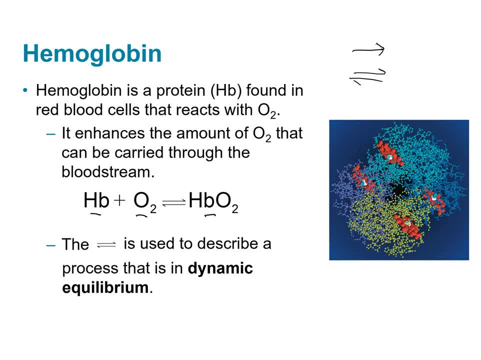 Where we have a forward reaction with the arrow pointed over to our right, And then we have the reverse reaction, With the arrow pointed towards our left. And the reason this is important is because not only does hemoglobin and oxygen bind to form the product oxygenated hemoglobin, 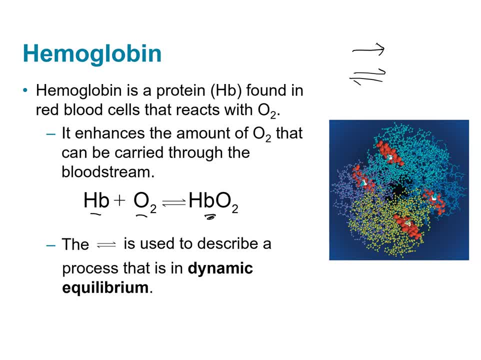 But oxygenated hemoglobin can dissociate in the reverse direction, releasing oxygen and liberating nonoxygenated hemoglobin. So what we're really looking at is a dynamic forward and reverse reaction Which our biology utilizes to its advantage. So let's talk about that a little bit. 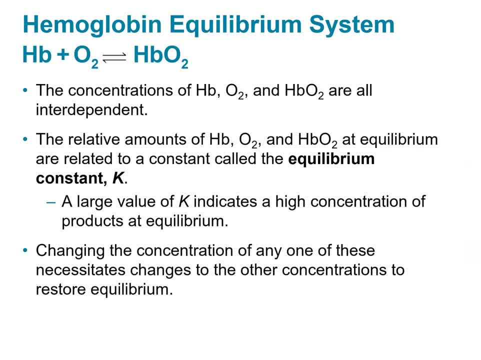 So the concentrations of our hemoglobin, oxygen and oxyhemoglobin are all interdependent And the ratios of all of these depend on how much is available of the others. So the way we describe this In terms of modeling is with the equilibrium constant. 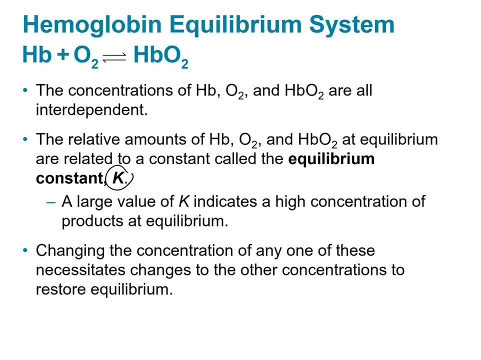 Which is K. So this term K is our equilibrium constant And generally some rules that we want to get comfortable with right out the gate. If you have a large value for K, That means that the products at equilibrium are in fairly high concentrations. 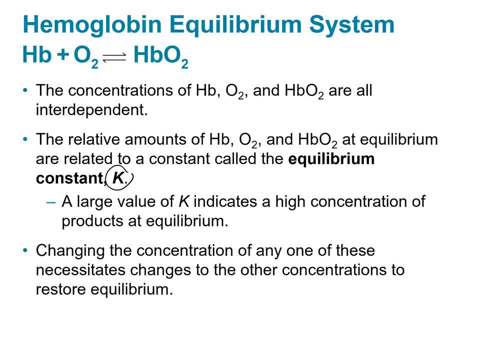 And if you have low values for K, That means your products are going to be in low concentrations At equilibrium And we're going to spend a lot of time reinforcing this concept. But just to kind of get the discussion started, That's where we're at. 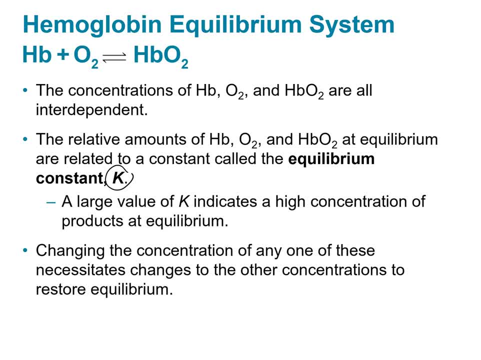 And what's really important to note Is that if you change the concentration of any of our reactants or products in equilibrium reaction, That's going to necessitate a change to the concentrations of the other components To return everything to equilibrium. So to that constant K. 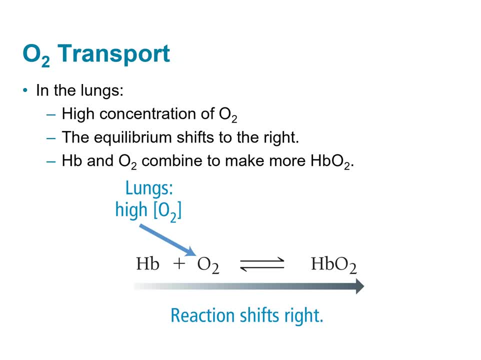 So a good example of this would be oxygen transport with hemoglobin, So in the lungs, Where we have very high concentrations of oxygen available. What happens is Is in our reaction that we're looking at down here at the bottom, We are adding oxygen to our equilibrium system. 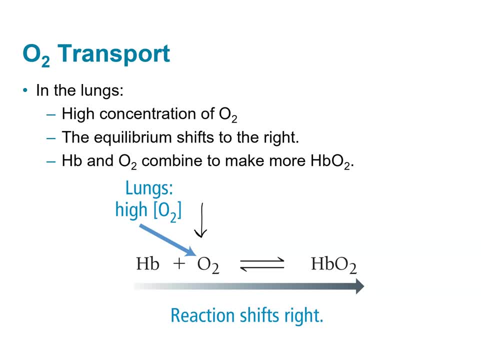 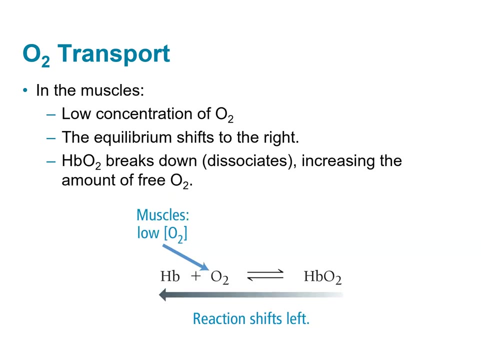 And what this does Is to make everything return to equilibrium, Drives the reaction Towards oxyhemoglobin. However, once that oxyhemoglobin reaches areas of low oxygen concentration, Such as in the muscles, We are, The muscles are consuming this oxygen. 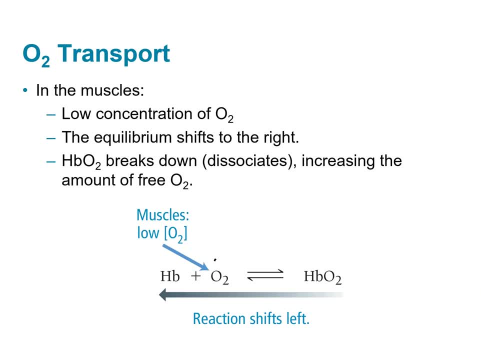 We don't have enough of it around, So these levels are decreasing Or being removed from the system. And as this is being removed from the system To return to equilibrium, Our reaction gets pulled Over towards the reactant side, And this is happening. 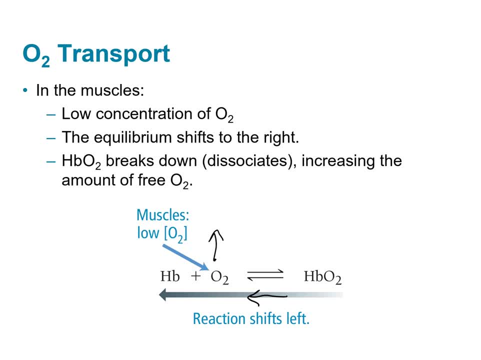 Through an active dissociation of the oxyhemoglobin back to our Standard hemoglobin and free oxygen, And this is how oxyhemoglobin liberates oxygen into tissues that need it. Another fun variation on this theme Is the fact that we have different types of hemoglobin. 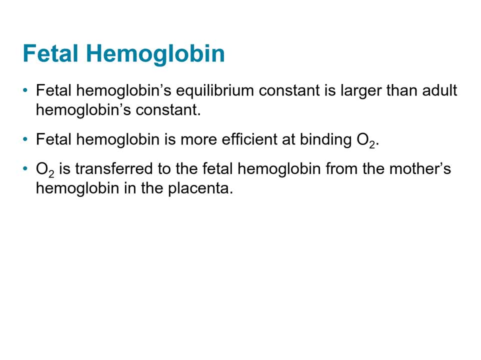 So fetal hemoglobin Has a higher affinity For oxygen Than adult hemoglobin And this is super important Because we want the fetus In a developing Environment to have preference For oxygen. So how that works is fetal hemoglobin. 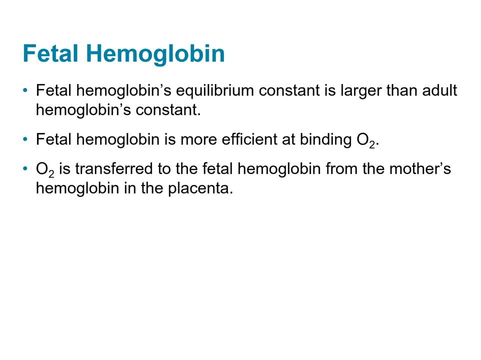 Equilibrium constant Is larger than the adult hemoglobin, And this makes it more efficient At binding oxygen And pushing the reaction Towards oxyhemoglobin, And then This also facilitates the transfer Of oxygen From the mother's hemoglobin. 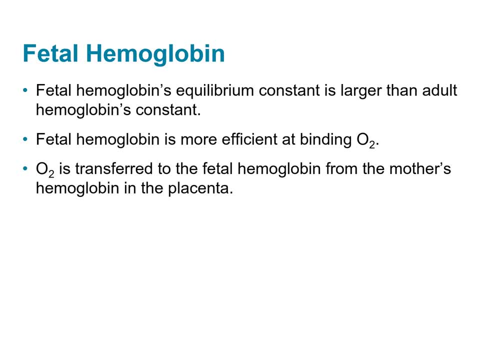 To the fetal hemoglobin- Nice little survival mechanism. Likewise we also see- And this isn't in the book- Variations in hemoglobin and myoglobin In aquatic mammals That need to be under water For long periods of time, And you also see changes. 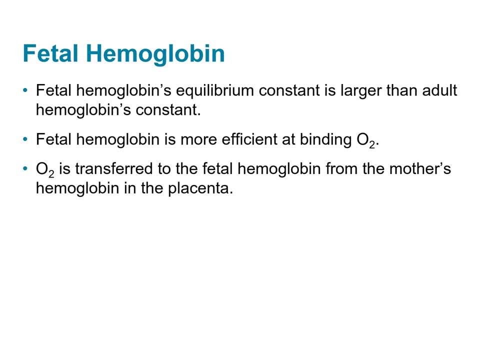 To the hemoglobin and myoglobin structures In reptiles that are under water For long periods of time. They change their K values, The equilibrium constants, So that Their hemoglobin and myoglobin Is perfectly tuned to the environment In which they need to be competitive. 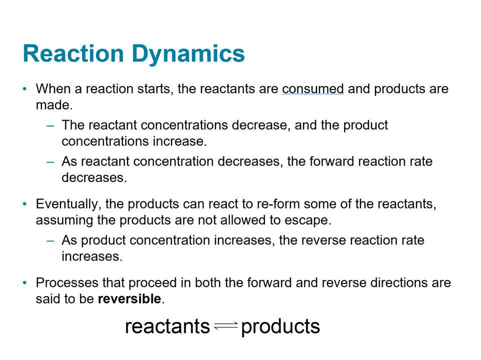 So, moving along from the hemoglobin, We can start to really dive into What equilibrium is. So when a reaction starts, Reactants are consumed And products are formed Right. So in any general reaction We're going to have A equivalence of A. 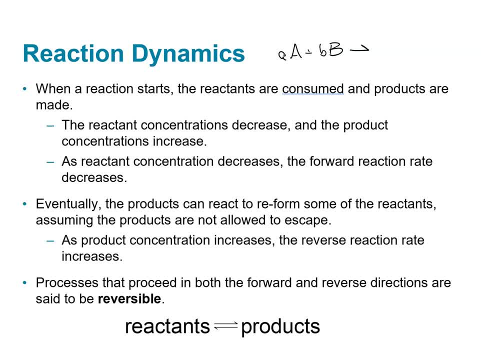 Plus B equivalence of B In a reversible reaction form. C equivalence of C. Plus D equivalence of D. Let me see if I can get those pluses To look more like plus signs. Apologies for terrible plus signs. So on this side, 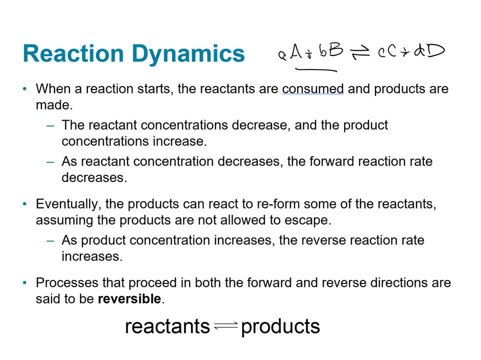 We have our reactants And the initiation of a reaction, Because we have no products yet. So that's what we're really starting with here: Reactants start to come together And the reaction single-sidedly Moves towards our products. Now 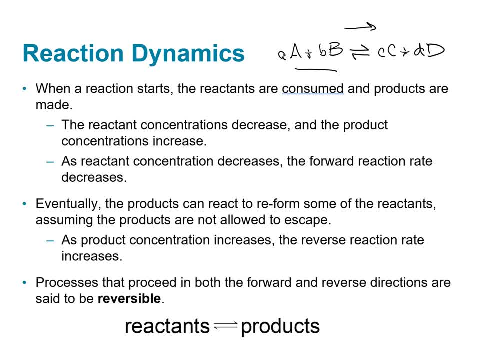 As our concentration of our reactants Decrease, The rate of that forward reaction Also decreases, Because rate of reaction is dependent on concentration. So as we're consuming our reactants, The speed with which we consume them Decreases Likewise. 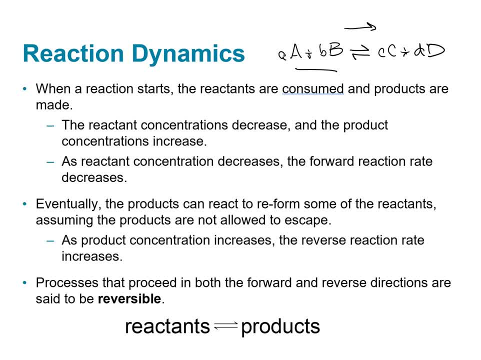 As we form products, The products Start to Have the ability to do the reverse reaction, And the reverse reaction Is this dissociation Of the products Back to our reactants And, as we build up the concentration of products, The rate of the reverse reaction. 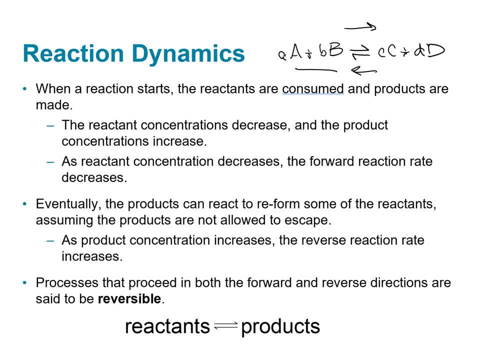 Will increase Because we're increasing the concentration Of the products. So What you end up with Is: at some point The process is proceed At the same rate When the forward reaction rate of reaction And the reverse reaction rate of reaction. 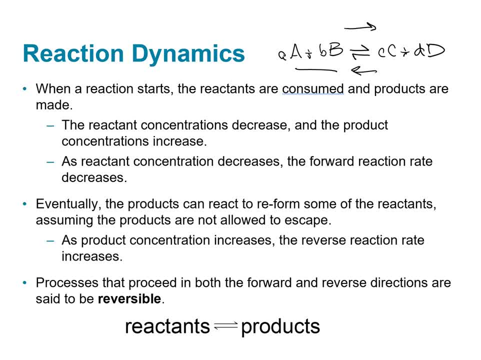 Equal one another When the reactions happening at this speed, At the same reaction. This way, You reach what Is called equilibrium Right. So that's what we're going to be studying And That's the general concept. To remember is that. 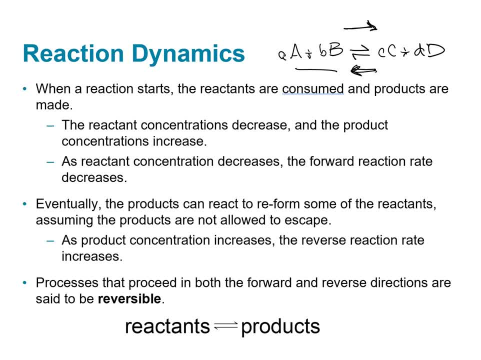 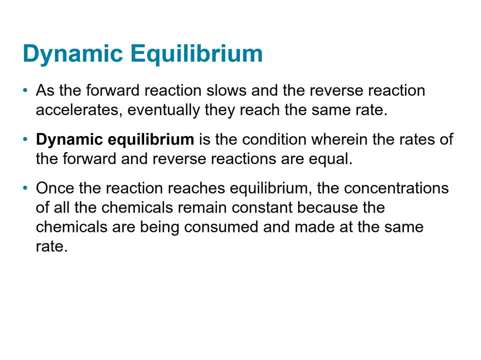 The relative forward rate of reaction And relative reverse rate of reaction Are what going to determine The relative quantities Of product and reactant. So Dynamic equilibrium. Dynamic equilibrium Is the condition wherein The rates of forward and reverse reactions are equal. 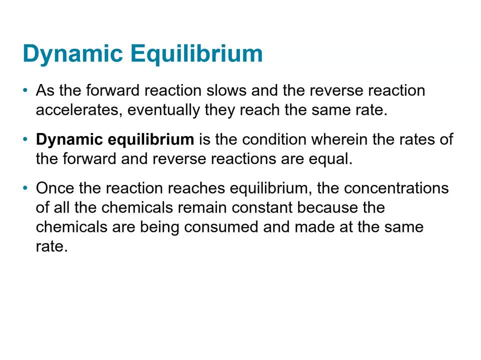 Basically- just a nice way to restate What we just said- When the rates of forward and reverse reaction Equal each other At dynamic equilibrium- And it's important to remember That it's dynamic Because we continuously have reaction taking place- 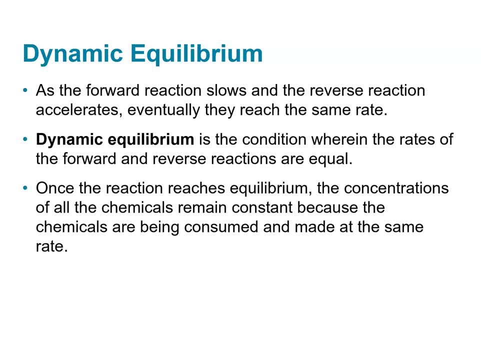 It's just that the concentrations aren't changing Because the rate of forward And rate of reverse reaction Are the same, Doesn't mean that chemically everything is static, Just the concentrations. And doesn't mean we can't change the concentrations. 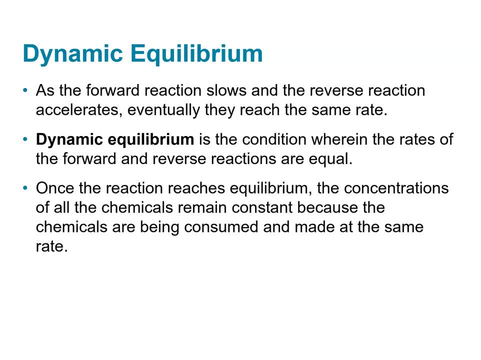 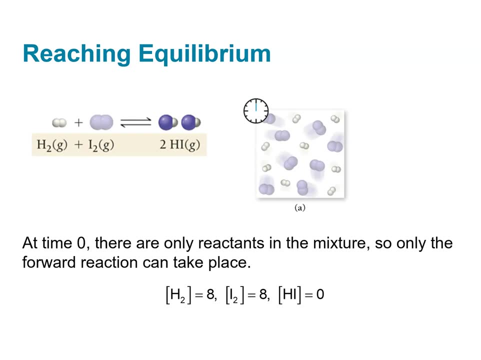 By modifying the system Or reaction conditions To shift the equilibrium conditions. So once the reaction Is at this equilibrium, The concentrations of all of our chemicals Remain constant, And that's what is our constant, But everything else is still chemically in motion. 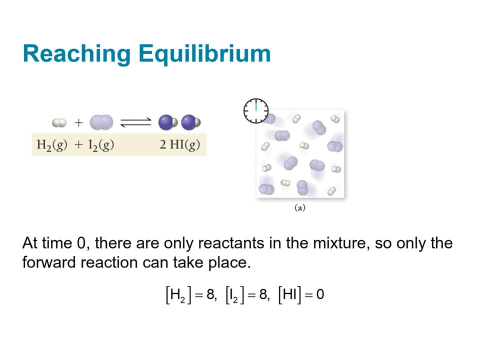 So a good example of this Process. pictorially, We have the reaction Of hydrogen gas and iodine gas, Reversibly forming Two equivalents of hydrogen, iodine Or hydroiodic acid gas. So at time zero, The initiation of this reaction, 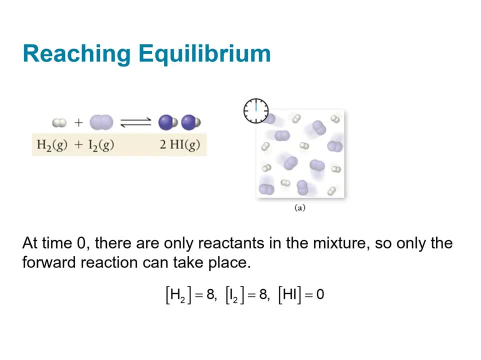 We put the hydrogen iodine together In order to react with one another. So in this particular case, Arbitrarily, we've set the reaction Concentrations of both Hydrogen and iodine gas To eight moles per liter. 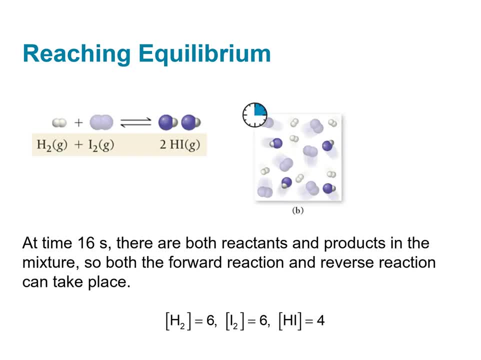 And the concentration Of the product is zero. Moving forward In 16 seconds of the reaction, We've reduced our concentration of hydrogen and iodine From eight to six a piece And we've formed four moles, Or, excuse me. 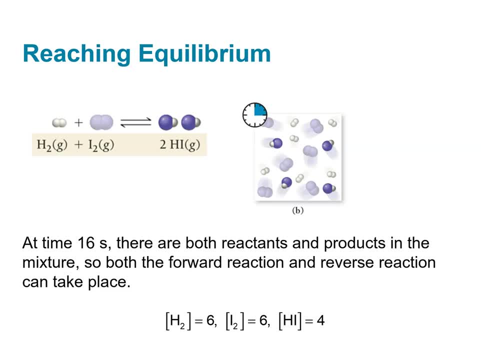 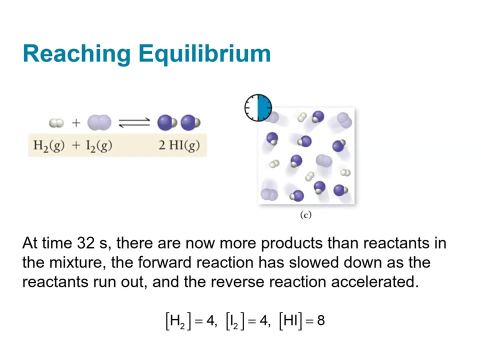 Four moles per liter Hydrogen iodine gas. At this point, though, Hydrogen iodine gas Is also Proceeding in the reverse direction, And this is going to slow the reaction Of hydrogen and iodine, And at 32 seconds. 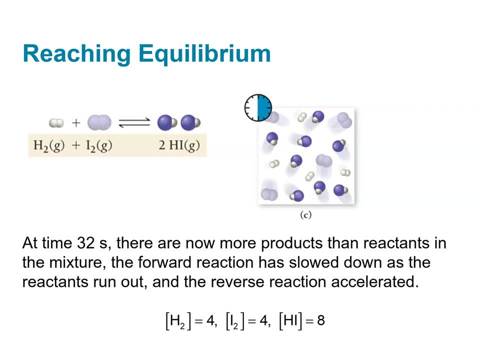 We have A even further reduced concentration Of hydrogen and iodine, Now at four moles per liter a piece Instead of where we started at eight. The concentration of the hydrogen iodine Is now at eight moles per liter, And if we 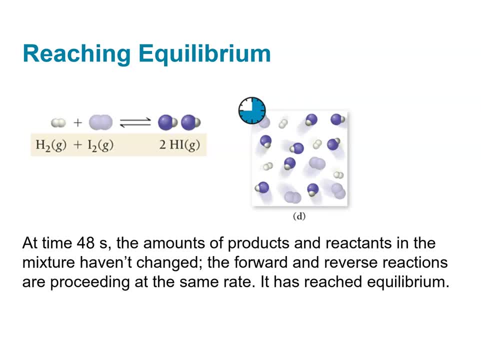 Sit around a little bit longer, We realize that the concentration Hasn't changed at all From the previous set of conditions, And this is because the forward rate of reaction And the reverse rate of reaction Are the same, meaning The speed at which. 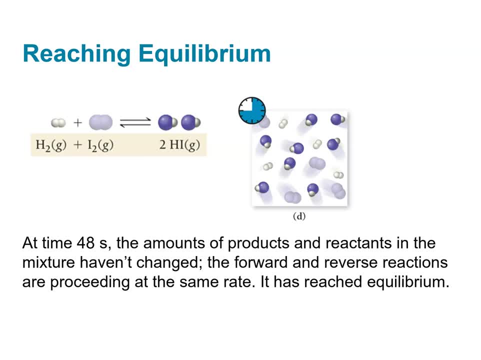 At those concentrations. We thought 32 seconds in the previous slide At those concentrations. The forward rate of reaction Of the hydrogen iodine to form Two equivalents of hydrogen iodide Is identical to the reverse reaction Of the dissociation. 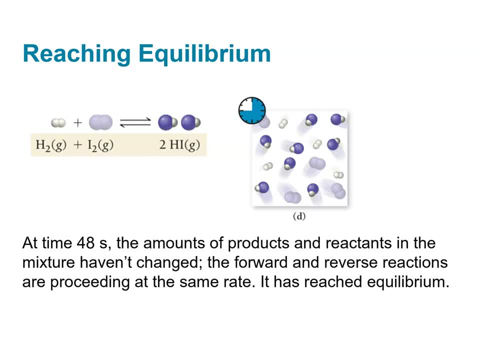 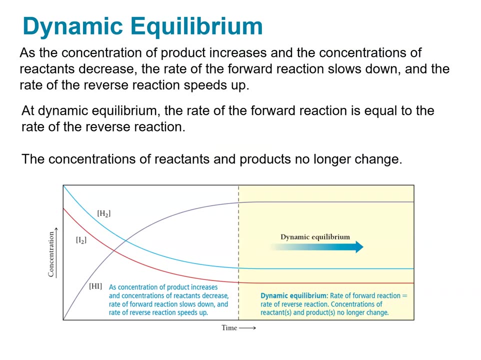 Of two equivalents of hydrogen iodide To One equivalent of hydrogen gas And one equivalent of iodine gas. Now we have a dynamic equilibrium system, And this is just a Nice pictorial way To look at what We just said. 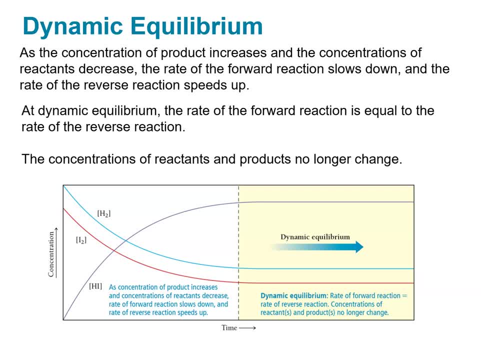 And it's just nice Graphical representation of it. So What we can look at here initially Is we have Our concentration of iodine Gas, Our concentration of hydrogen gas, In red and blue respectively, And then with the purple line. 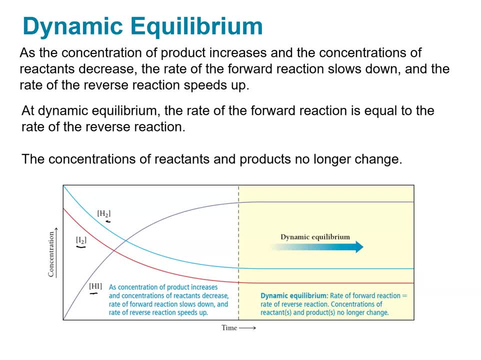 We have our product, Hydrogen iodide, And right out the gate You can see as the reaction starts, Rate of reaction decrease As their concentrations decrease And then the rate of reaction Or the concentration Of hydrogen iodide Increases. 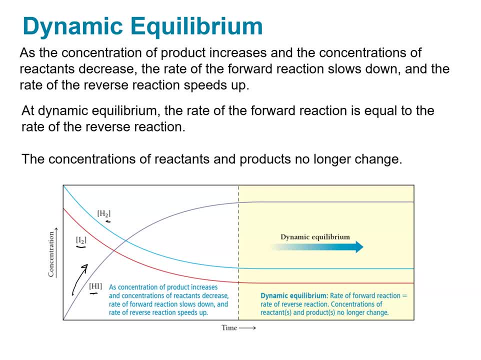 Here, As the reaction proceeds And as these Slow, The rate of reaction slows And flatten out, We reach equilibrium Where everything, following this time of reaching equilibrium, The concentrations, are maintained For all of our reactants And Products. 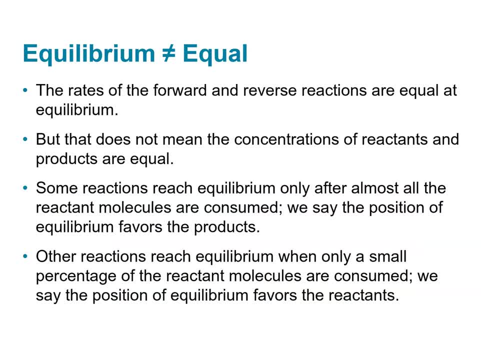 So One thing that's really important To remember: Equilibrium does not mean equal, Doesn't mean that there's any equality In the concentrations of our reactants Or our products. It means that There's a balance In the rate of reaction. 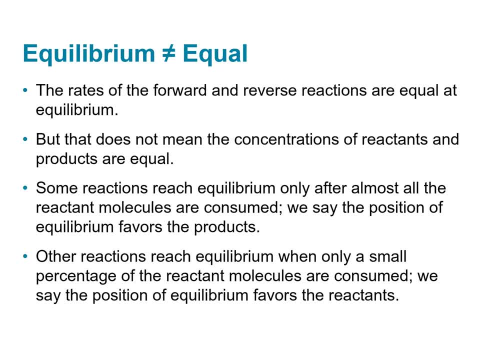 Forward and the rate of reaction In reverse, And the rate of reaction itself Can be very, very different, Because some reactions are highly favorable, Where the products are highly favored. Some reactions- The products are not favored, The reactants are favored. 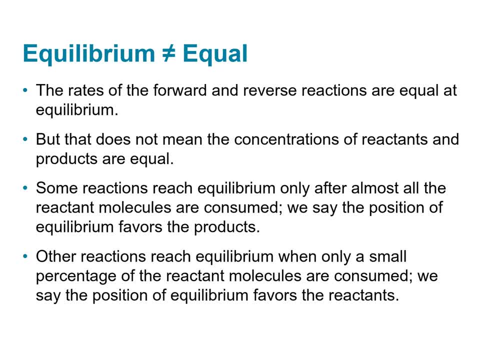 And only a small amount of product is formed. So It's not equal, It's just in equilibrium. So For these different scenarios I just talked about, After nearly all of the reactants Are consumed, And in that particular case, 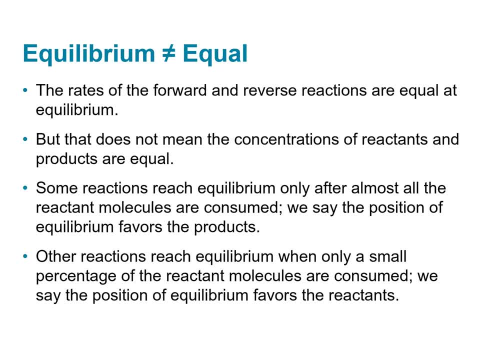 We say that equilibrium favors products. And the other scenario That we talked about: The reaction can reach equilibrium When just a very small percent Of reactant molecules are consumed, And under those scenarios We say that equilibrium favors reactants. So how do we numerically, 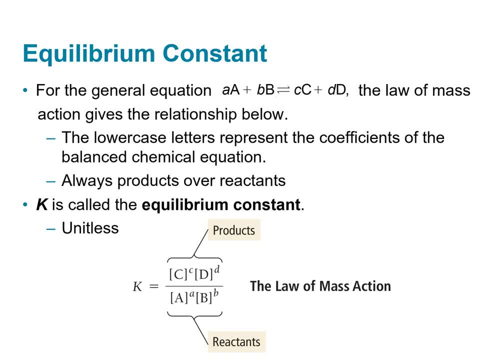 Assess The equilibrium constant. So for this general reaction I poorly wrote out On one of the earlier slides, We have this general expression For generic reaction Where A units of A Plus B units of B, With both A and B being our reactants. 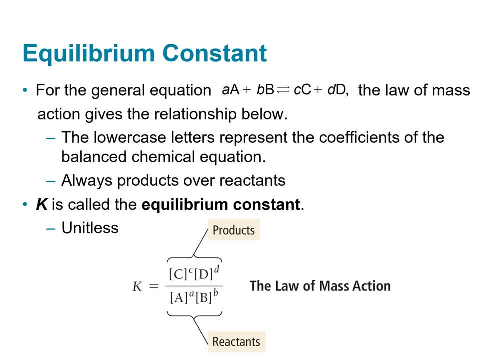 Are in equilibrium, With C units of C Plus D units of D, With C and D Being our products, And The lower case letters Of A, B, C and D Are all our molar coefficients Of our reaction. 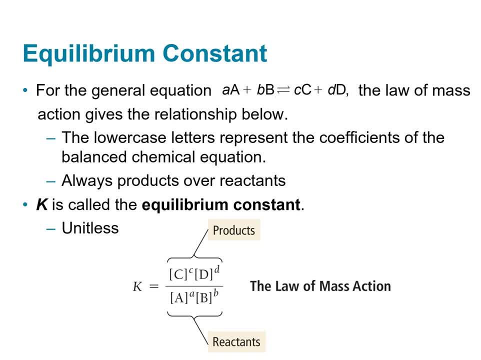 In our balanced equation And our identities, Of our components Or our capitals. Now, when we set up The law of mass action, Which we see in this equation on the bottom, Which is the relationship Of products over reactants, We always put products over reactants. 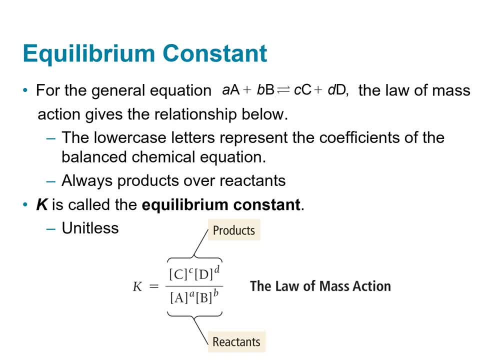 Always In equilibrium. It's always, always, always. Products over reactants. Say it out loud to yourself When you're doing your homework: Products over reactants. That's the relationship that matters When we're discussing equilibrium: Always. 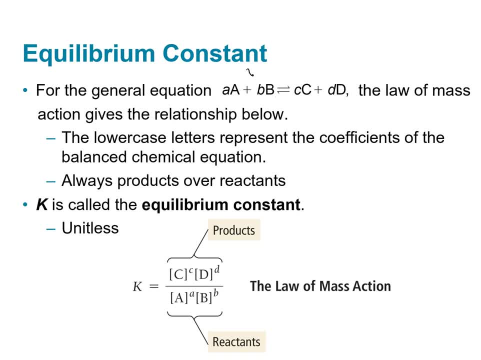 Now it's always as drawn. So because we've drawn it With A and B On the reactant side, That's our reactant side, And because C and D, We can just flip these around. C and D can be on the reactant side. 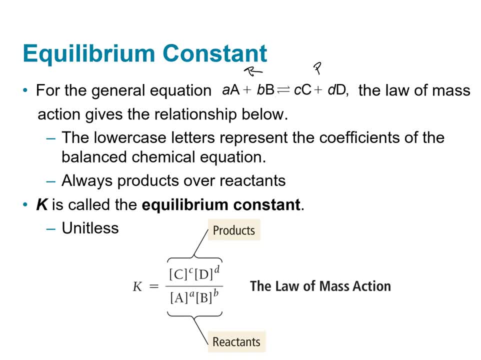 And A and B can be on the product side, And that changes the equilibrium constant, Obviously. So it's always As the reaction is written, With products being The components on the right side And the reactants being On the left side of the reaction. 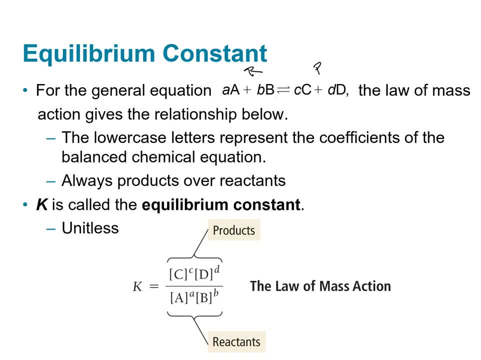 As written. And If we look at our law of mass action down here, We see that If you take the concentration of C Raised to its molar coefficient Times the concentration of D Raised to its molar coefficient And divide that, 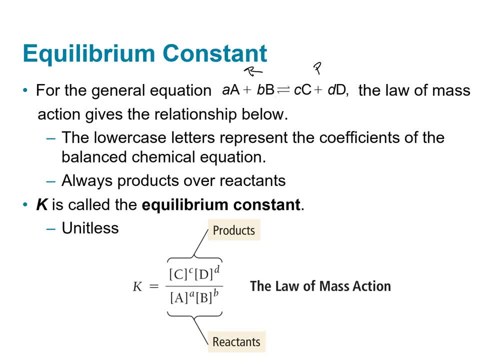 By the concentration of A Raised to its molar coefficient And B Raised to its coefficient. That gives us our equilibrium constant K, Which is unitless Because all the units from our concentrations Cancel one another in this particular scenario. Now, 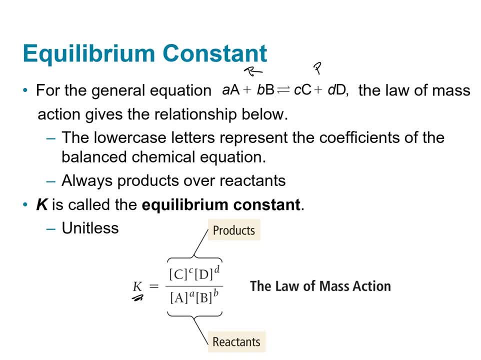 What I want to hammer Over and over and over Throughout this chapter- Not only products over reactants, But what K is an expression of Because of this relationship- Is, functionally, It's a ratio Of our products to our reactants. 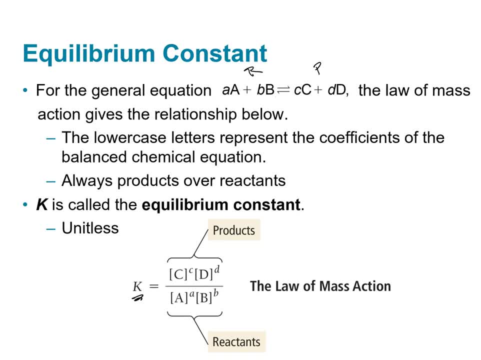 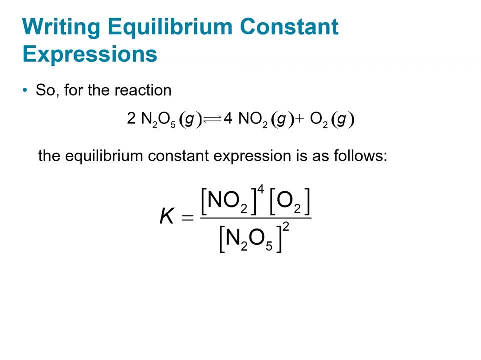 It's telling us How much products are favored Over our reactants, Or how favored our reactants are over our products, Based on the magnitude of its value. So Let's take a couple of these And just kind of get comfortable. 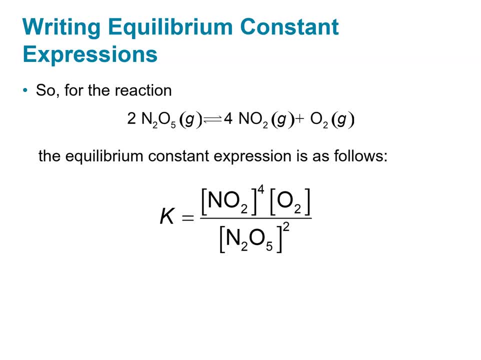 With the expression. So for this reaction, where we have Dinitrogen pentoxide, Two equivalents of it Are in equilibrium with four equivalents Of nitrogen dioxide Plus one equivalent of oxygen gas. To do this equilibrium expression We would first go right to: 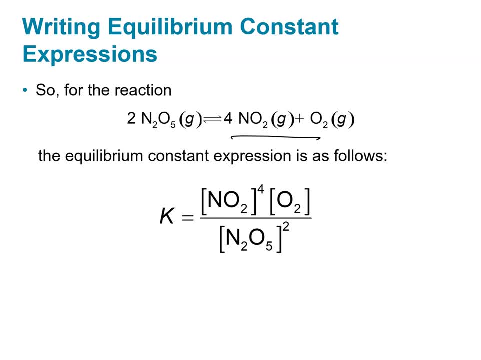 Our products Which are over here, And I would say the concentration Of nitrogen dioxide Raised to its molar coefficient, four Times the concentration of oxygen Raised to its molar coefficient of one, Which falls off the equation Because it's implied. 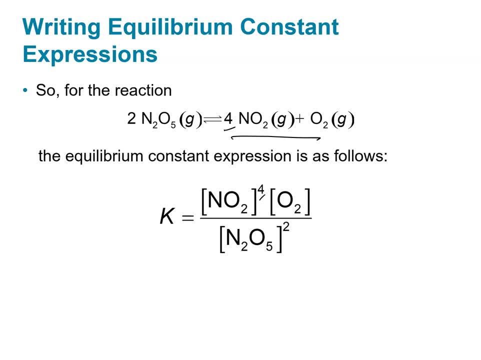 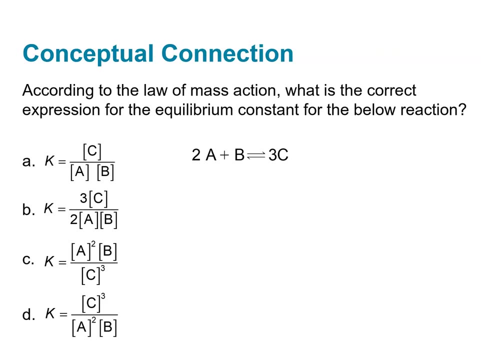 Divided by The concentration Of the reactant Dinitrogen pentoxide Raised to its molar coefficient two, Is going to give us our equilibrium Constant K. So as a conceptual check in, Let's go ahead and run this really fast. 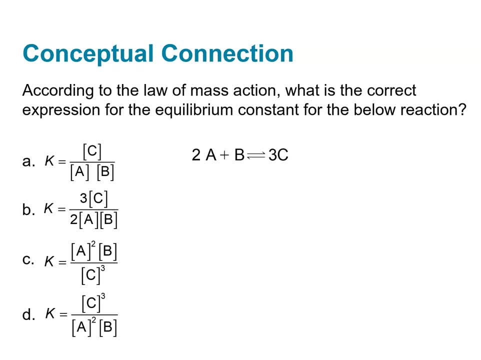 I think you guys will all be pretty proficient at it. Let's say we have the generic reaction: Two equivalents of reactant A Plus one equivalent of reactant B Are in equilibrium With three equivalents of product C. What would be? 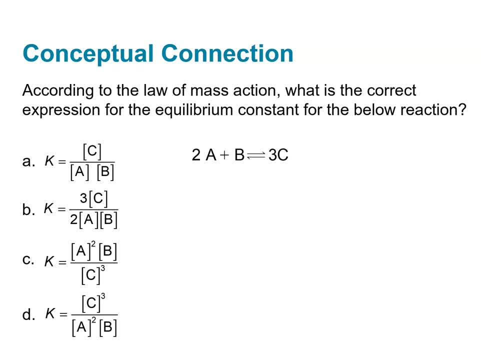 A Correct equilibrium expression To find K In this particular scenario. Well, Let's work it. I'm going to say K Is equal to The concentration of product C Raised to the third power, Because that's its molar coefficient. 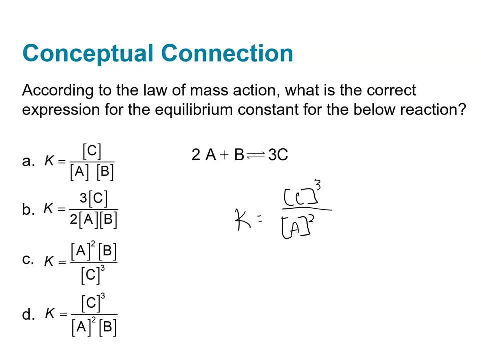 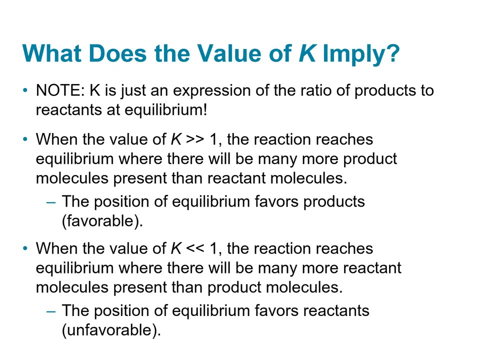 Divided by: Reactant A Is concentration squared Times reactant B Is concentration, So it should be, Should be D, And that's the correct answer. So what does K mean? Well, I've already kind of said That K is fundamentally. 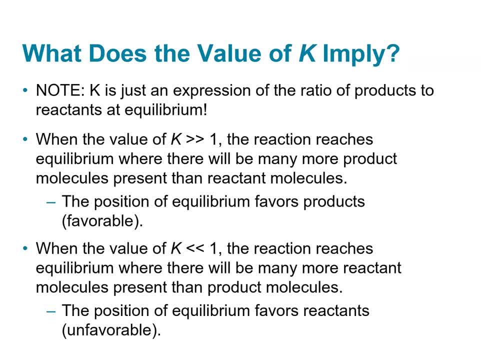 Fundamentally, K is just A ratio of products to reaction Reactants at equilibrium, Which means If K is substantially greater than one, That means that the amount of reactant Or, excuse me, products Is substantially more. Because if you have 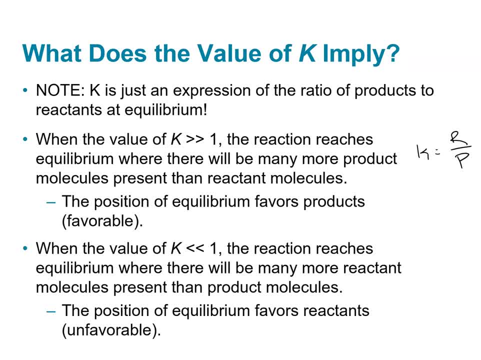 Let's say reactants over products Terms. If you have a large value over one, That means reactants Is going to be favored over products. In a small decimal state That's going to make K even larger Because you're dividing by something with a decimal. 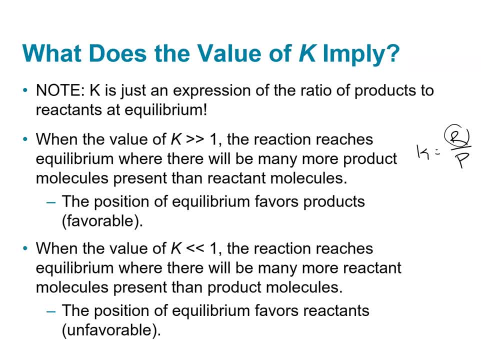 So when K is much larger than one, That means That when the reaction Reaches equilibrium, There's going to be much, much more. I'm sorry I drew this completely backwards Because of Products are always over reactants Excellent. 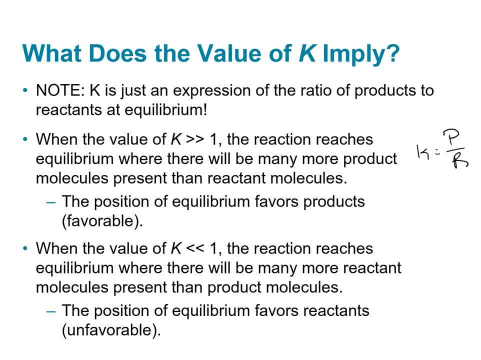 The products are going to be highly, highly, highly favored. Opposite of that scenario: If K is very small, Is much less than one, That means that the reactants Are going to be highly favored. Going back to one of our earlier slides, 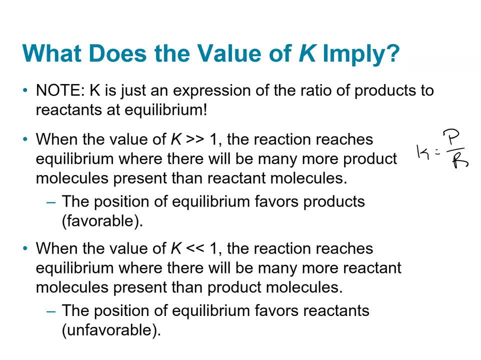 The other way we could say this: If Products are favored, That means the reaction is favorable. If reactants are highly favored Because K is very small, That means the reaction is unfavorable. The reaction does not proceed Towards products. as written. 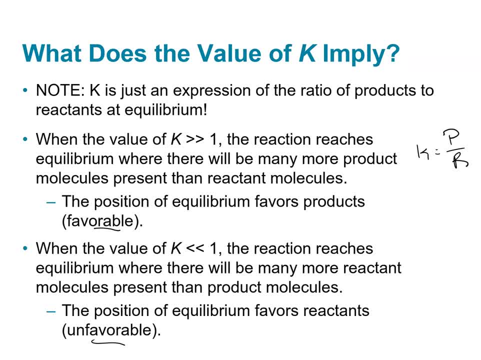 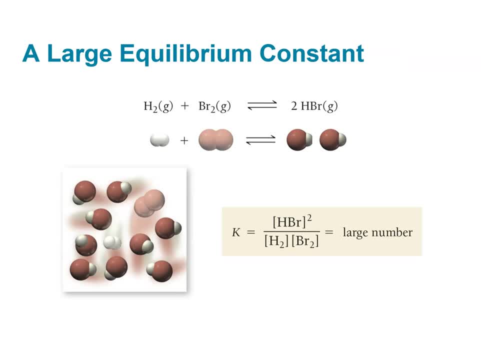 It predominantly Stays As reactants. So A couple pictorial examples of this. If we have a very large Equilibrium constant, Say the example here Where you have hydrogen gas Reacting with bromine gas, Forming hydrobromic acid, 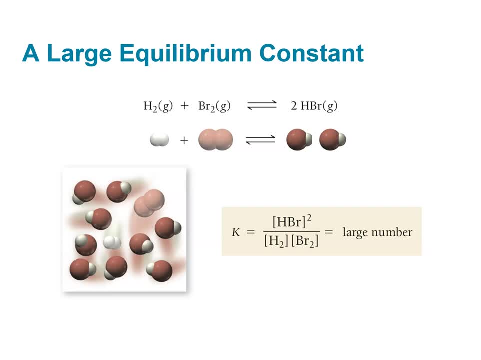 For two equivalents of hydrobromic acid In equilibrium. Most of This is going to proceed Towards products, Because The rate of reaction forward Is substantially higher Than the rate of reaction reverse- Another way to think of this. 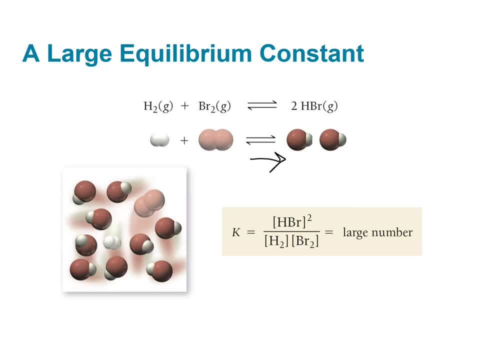 Is that It is much more favorable For the reactants, hydrogen bromine, To form hydrobromic acid Than for hydrobromic acid To decompose In the opposite fashion, Forming Hydrogen and bromine. 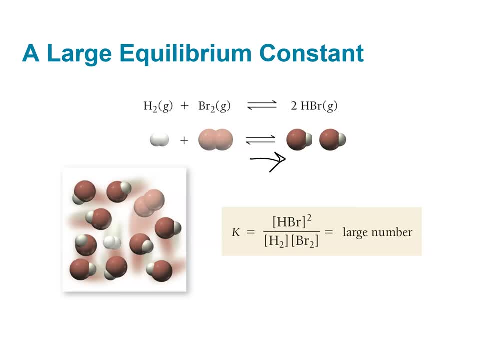 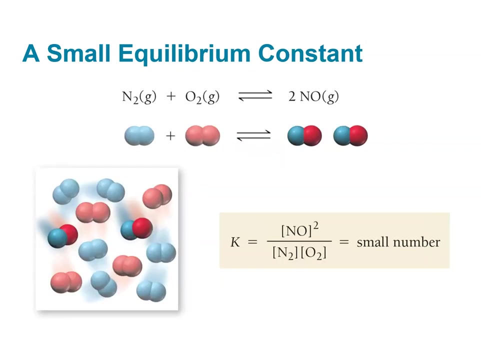 So because of this, We have much more Hydrobromic acid, Which you can see in this example With the pictures, And that is going to Make for a much larger term On top, A very small term On the bottom, 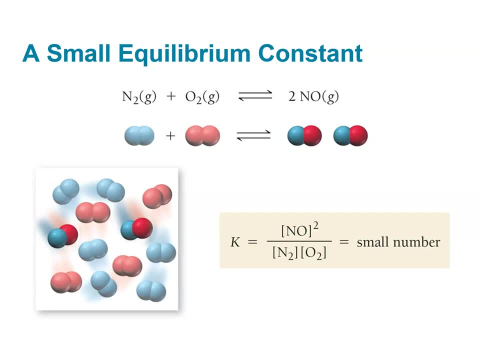 And that will give us A very large value for K. Opposite of this, If you put nitrogen gas And oxygen gas together In a reversible reaction Is not very favorable. Nitrogen and oxygen Don't particularly like to form. 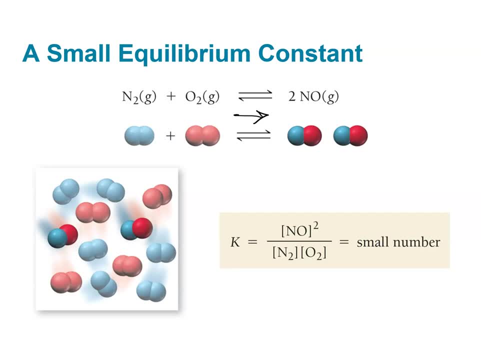 Nitrogen monoxide. However, Nitrogen monoxide Is perfectly fine Decomposing to form the more stable Nitrogen and oxygen gases. So because of this, Reactants are favored In this particular circumstance Instead of reactions, And because of that, 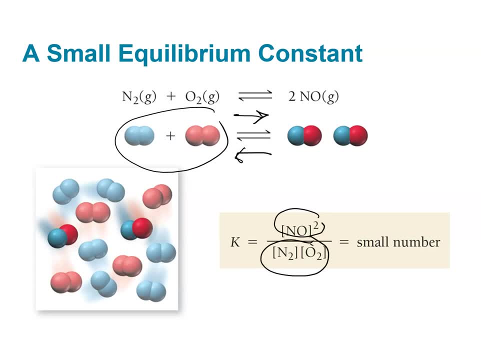 We have a fairly large value For our product And a fairly large value For our reactants And that is going to lead to a small K. So whenever you have a small K, That means remember That products are not favored. 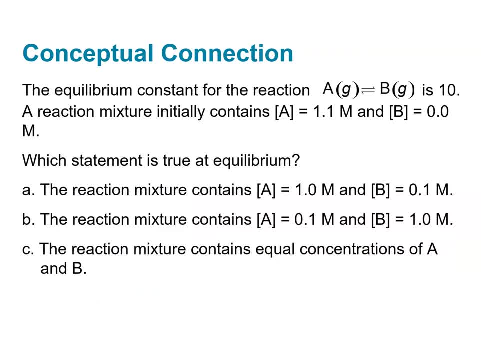 Reactants are favored. Alright, So let's do another conceptual connection problem here. The equilibrium constant For the reaction- A is in equilibrium with B- Is 10.. So K equals 10.. The reaction mixture initially contains 1.1 moles per liter of A. 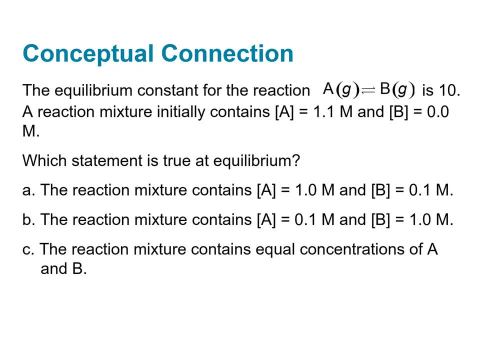 And no B. And this makes sense because If you just have A Going towards B Under initial reaction conditions, You won't have any B forming But at equilibrium. Which of these could be True if K is 10.? The reaction mixture contains: 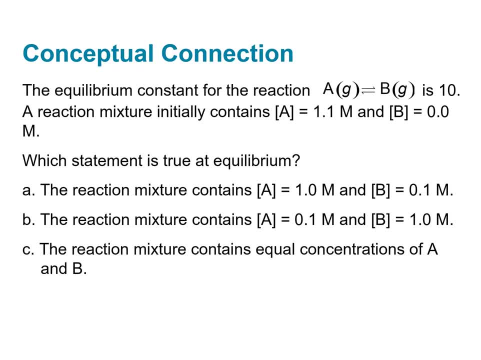 A at 1 mole per liter And B at 0.1 mole per liter Or B. The reaction mixture contains A at 0.1 moles per liter And B at 1 mole per liter Or C. The reaction concentrations are equal. 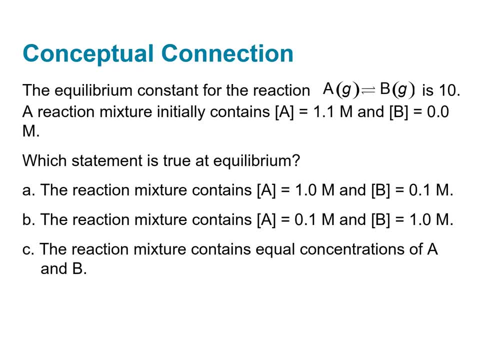 So we know right away: The reaction concentrations are not equal, Because K equals 10. Which means we have a 10 to 1. Ratio Of K Equals The concentration of B Over The concentration of A, Because products over reactants. 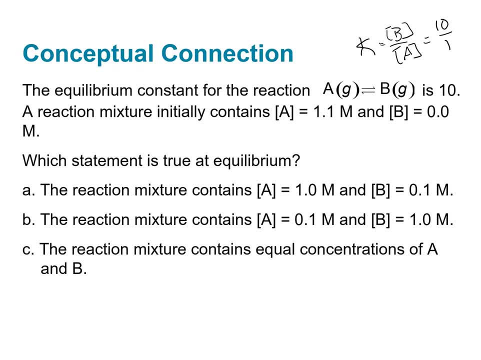 And if this is 10. That means you have a 10 to 1 ratio Of B to A In terms of molar ratio At equilibrium. So right away We know the number of moles can't change, So we have. 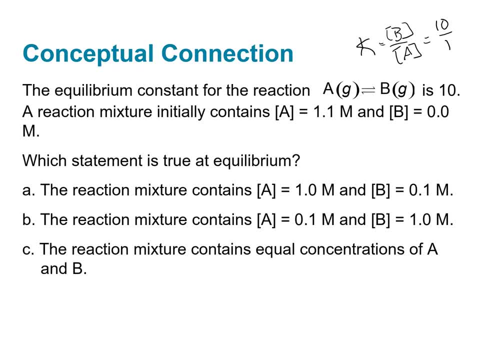 To. if we start with 1.1 moles And it's a 10 to 1 ratio, One is going to have 1 molar And one's going to have 0.1 molar concentration, But which one's which? 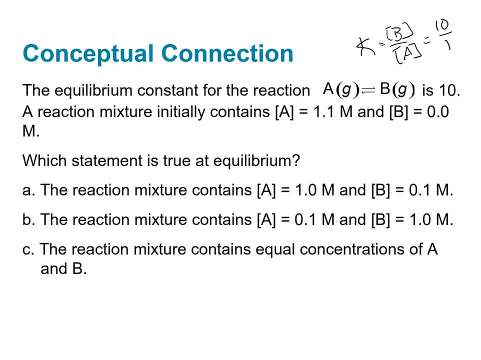 Well, we've already drawn it out: B, in this particular case, should have 10 times the concentration of A. So the scenario Of B being 1 molar And A being 0.1 molar would be correct. The answer should be B. 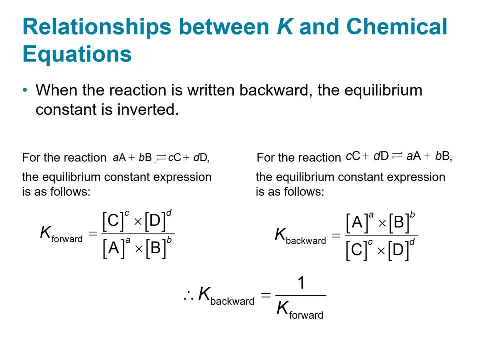 And in this case it is. So let's talk Through the relationships Between K And chemical equations. So when the reaction Is written backwards- Because I keep referring to As written- The equilibrium constant Is just inverted. These are basically. 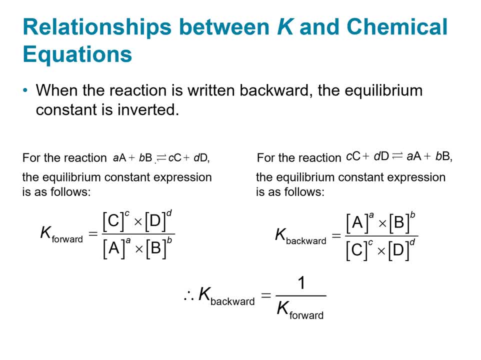 We're going to go through a series of shortcuts, Basic concepts on how K is manipulated When you change The way you're looking at your reaction. So if we have our generic reaction- A units of A Plus B units of B- 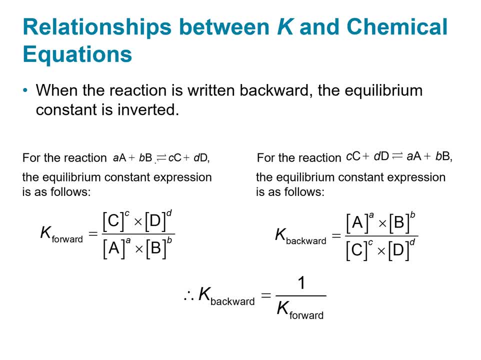 For our reactants are in equilibrium With C units of C Plus D units of D For our products. We would write the equilibrium expression For the forward reaction As drawn Here. So our equilibrium constant K Would be the concentration of C. 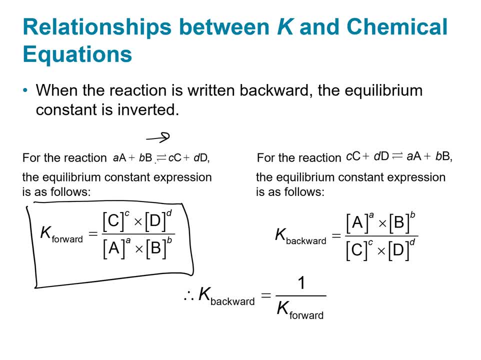 To C power times, the concentration of D To D power Times, the concentration of B To B power, Or just products over reactants. Now, if we were to look at it the opposite direction, Going from products To reactants, We would redraw this. 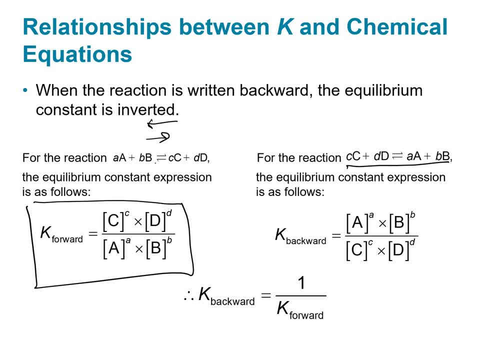 Here, With C plus D Going to equilibrium With A plus B. This is just the same reaction Being viewed from the opposite direction, And because of that We would write K As drawn here, With A and B As our product. 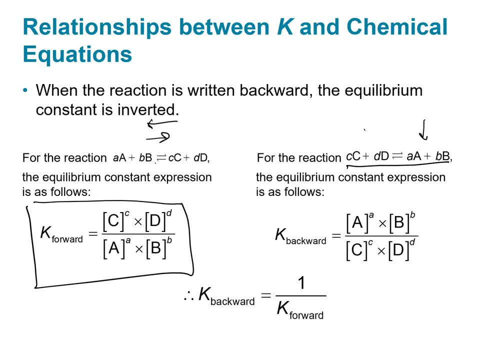 Because it is on the product side, And C and D Being on the reactant side. Now, The nice thing about this relationship Is that these are just the inverse of one another. So If you're looking for the reverse Of K, 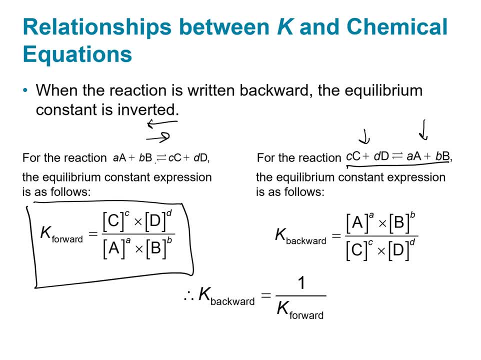 From the forward reaction. So let's say K for the forward reaction is Some arbitrary number. If you're interested in what the K is For the reverse reaction As drawn, It's just going to be one over K. So K backwards is just one over K forwards. 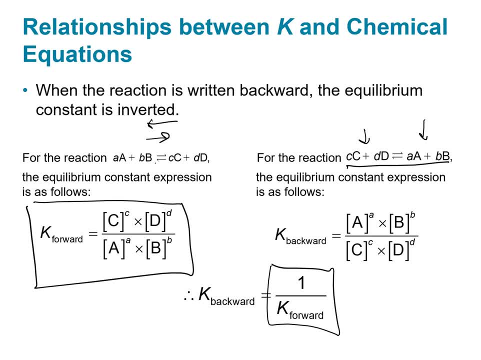 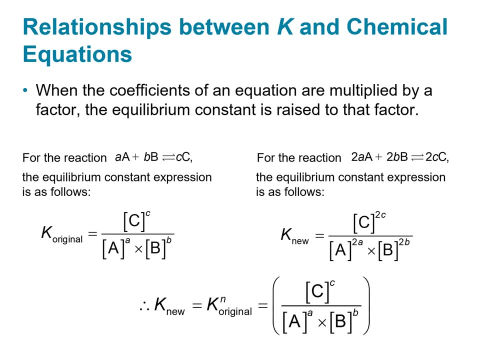 You can just take the invert of K If you're interested in what K is For the reverse of the reaction As drawn Pretty straight forward And it's going to save you a lot of time. Another relationship that's important When the coefficients of an equation 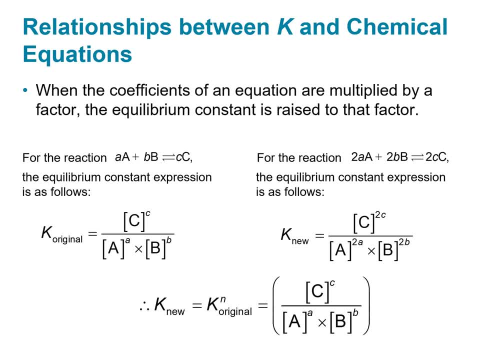 Are multiplied by a factor, The equilibrium constant Is raised to that factor. Pretty straight forward. So for the reaction A plus B is in equilibrium with C. We can draw An original expression, In this case K original, Where the product C. 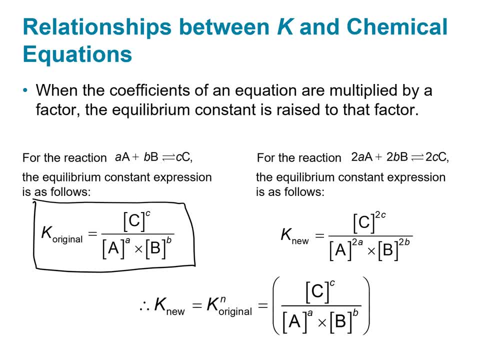 Raises C power over A to A power. Times B to B power, Gives us our original K. Now, If we raise everything To C Times two, Where we have two additional molar equivalents For two times the molar equivalents, 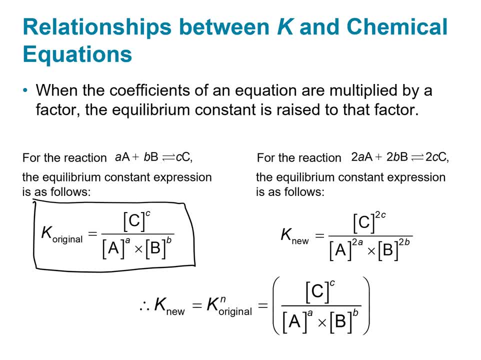 For all of these things, Where A and B and C all Have twice the molar concentrations, We could just sub in Those extra values To For all of these components, And What we'll find Is that the original term. 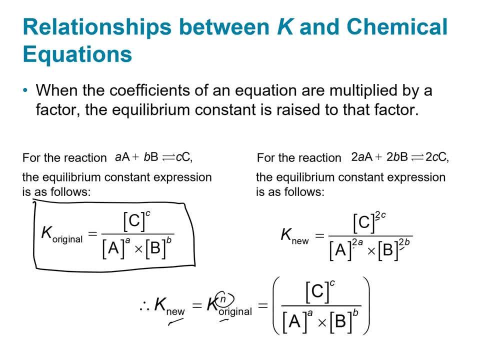 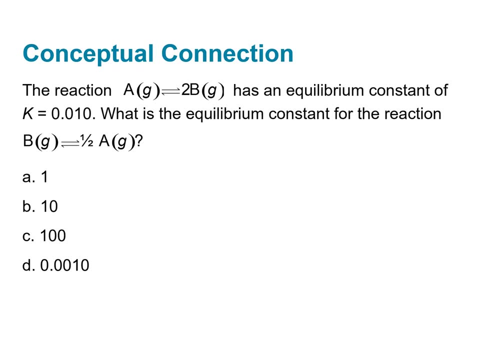 Will equal The equilibrium constant Raised to the square. Pretty straight forward, So let's do a quick check in With these. The reaction Of reactant A Being in equilibrium With two equivalents of Product B Has an equilibrium constant. 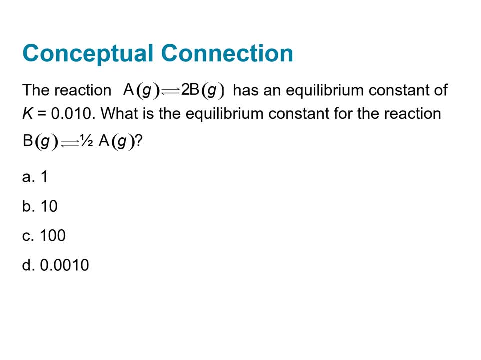 K equals 0.010.. Which is the equilibrium constant For the reaction. B Is in equilibrium with half of an equivalent of A. Well, What's really slick about this one Is that we can Immediately just do the reverse. 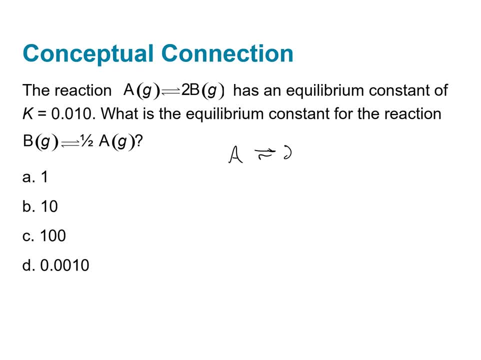 Let's say here A is in equilibrium With two, B Is functionally the same As one half of A Is in equilibrium with B, Because we're just dividing Both sides by two. And if we were to draw this in reverse? 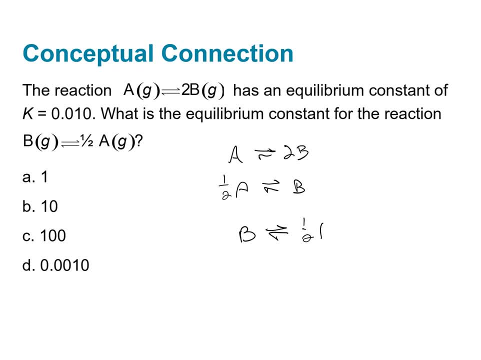 It would be. B Is in equilibrium with one half of A, So That's what we have really reached here. We've done two different transformations. Now, What's slick about this Is what is K as drawn forward? It's 0.010.. 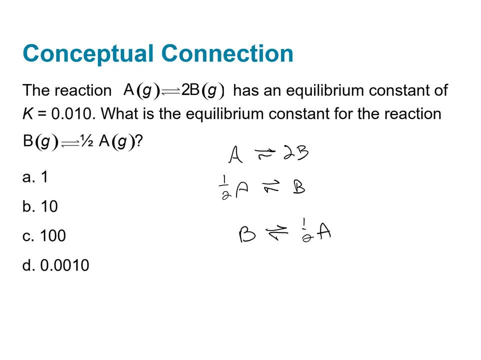 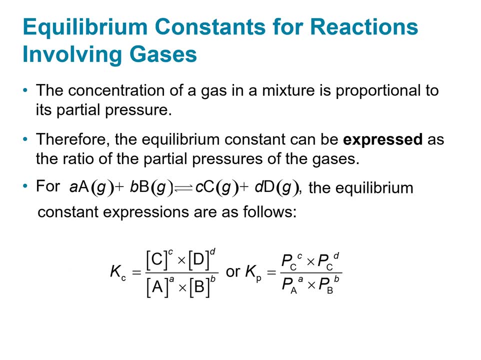 What's the invert of that? It's 10.. 10. And it is Nice, Okay. So, adding a layer of complexity to this, We can Determine equilibrium constant expressions From concentrations, Which is what we've been doing. 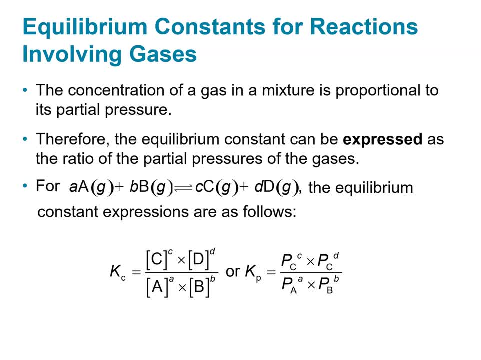 We can also, For gases, Use partial pressures Of the gas. So the concentration of a gas in a mixture Is proportional to its partial pressure. Once again, It's proportional to partial pressure. Therefore, it's okay To make equilibrium expressions. 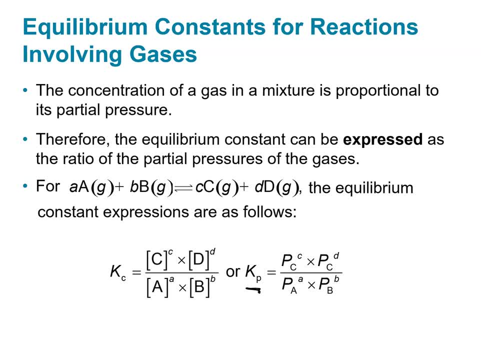 For K sub P Right here, As a ratio of partial pressures Of all of the gases Raised to their respective Molar equivalents. Now, This doesn't mean That the Concentration Determined value for K Is going to be the same. 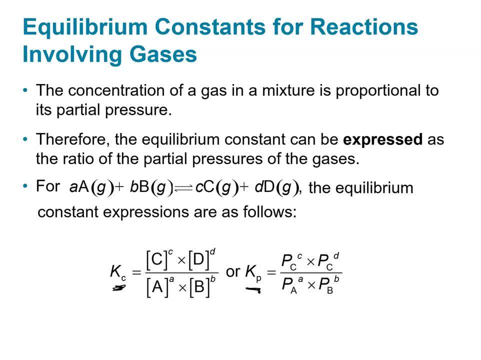 As the partial pressure Determination of K, But they're both valuable ways To look at equilibrium. Sometimes they're the same And the book gets into that a little bit, But just don't take for granted That they're going to be identical. 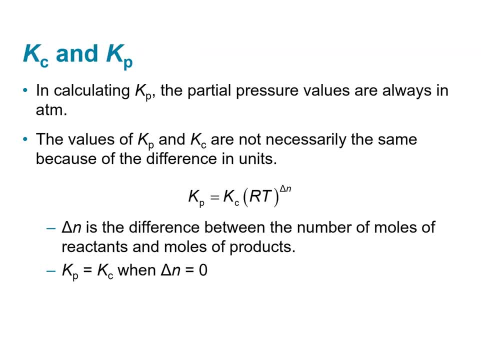 Look at equilibrium And gaseous systems. So let's look a little bit more At K sub C and K sub P. So in calculating the Equilibrium expression From partial pressures, The partial pressure values Are always in atmospheres. 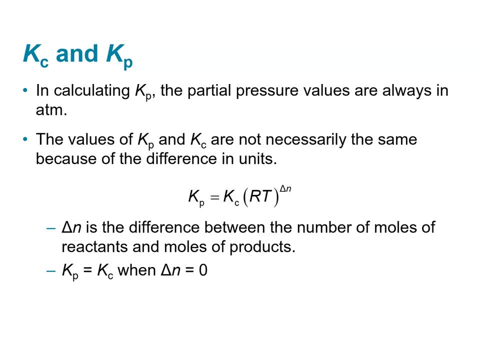 That's all very important. The value of the K From K sub P and K sub C Are not necessarily the same, Because they do have differences in units. So the relationship here Is going to give you The exact Interconversion between the two. 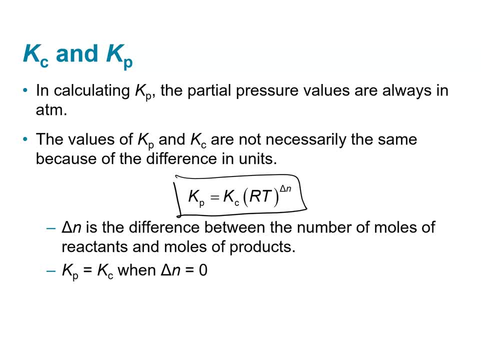 So if you're asked to Interconvert between the two And you have the temperature reaction, The number of moles that are changing And the ideal gas law constant, Which we do, You can determine this. Now, What's really important to note? 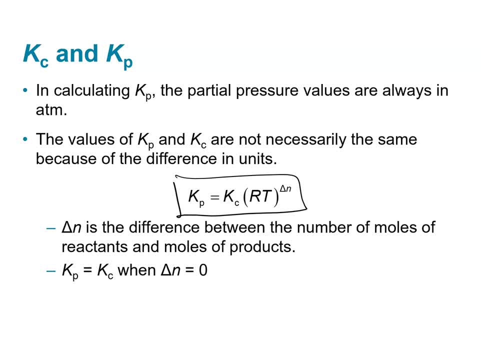 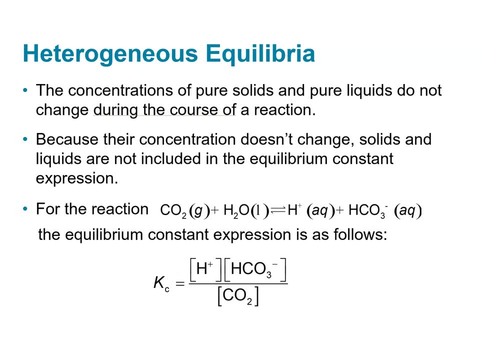 Is that if change in N is zero- That's the situation- K sub C are equivalent. Ooh, heterogeneous equilibrium. So This is one of the things that you have to go through When determining what matters And what doesn't matter. 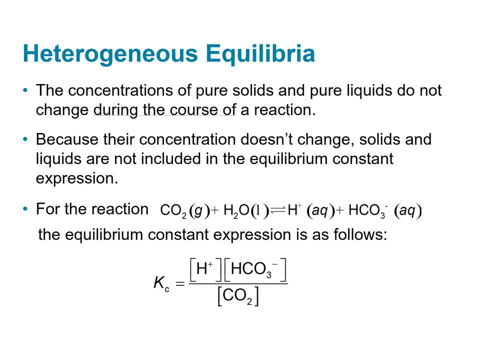 As part of Determining equilibrium concentrations. So We exclude concentrations Of pure solids and pure liquids From our equilibrium discussions, Because their concentrations Don't change over the course of reaction. What's the concentration of water In water? Does changing the amount of water? 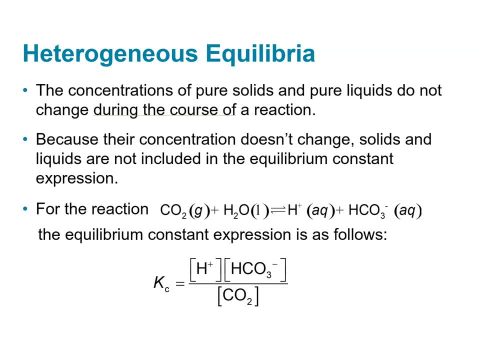 Change that concentration? No, it doesn't. Same thing for solids. If you have a pure solid, Let's say a pile of carbon, What's the concentration Of that pile of carbon? You can change its amount, But you don't fundamentally change its concentration. 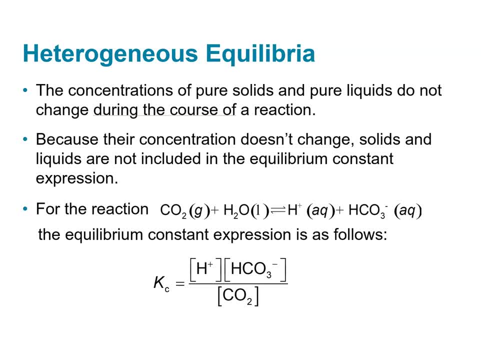 Because it's a pure solid. So instead of this, We can't look at changes of concentration As part of our equilibrium discussion. So a good example of this, Let's look at our third bullet. here We have Carbon dioxide gas. 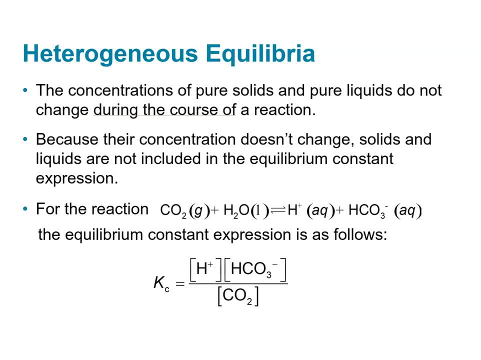 Reacting with liquid water Is in equilibrium To form free protons, And so One of the things For those of you who haven't had me before Is that hydrogen Has a proton And an electron, But no neutron. 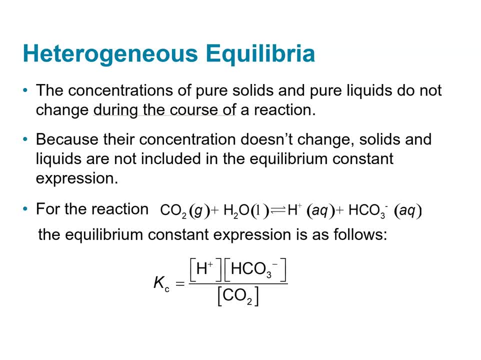 So if the hydrogen Loses its electron, It is literally a proton. So I will frequently refer to These H plus As a proton When I'm just discussing things. So if I say proton And you see H plus, That's what's going on. 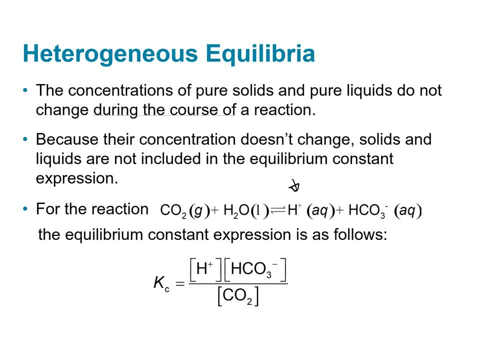 And so, Anyway, Coming back to this, We have carbon dioxide gas Reacting with liquid water In equilibrium With aqueous protons And HCO3 minus Also in aqueous phase. If we were to develop an equilibrium expression for this, 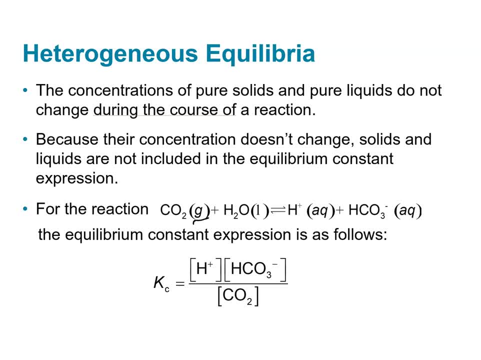 Based on concentrations. We would include The reactant CO2.. We would include the concentration of the product Of protons, Of our HCO3 minus, But we are excluding Anything to do With the concentration Of the liquid water. 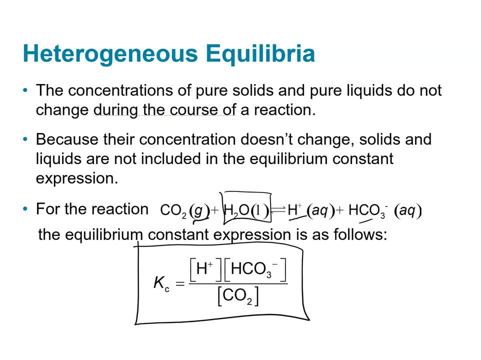 So our equilibrium expression Will look like this, Where we have our concentration of reactants Raised to their respective molar equivalents, Which are both one, in this case Divided by the concentration Of our product Reactant CO2 gas. 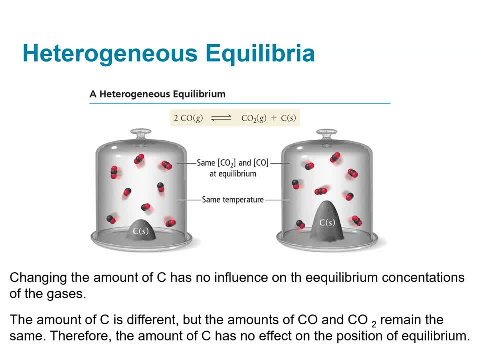 This Is a really nice little experiment, Kind of proving the point of what we just said, Because I know it's a bit of a head scratcher To say, well, if you have more something, How does that change the reaction? Well, let's take a look at. 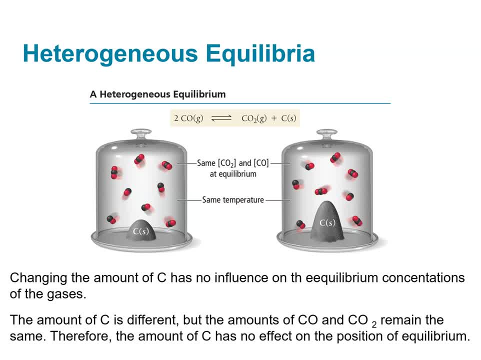 Equilibrium concentrations For reaction of Carbon monoxide gas, Which is our reactant here, In equilibrium with the products CO2 gas And solid carbon, So changing the amount of Solid carbon we have. In this case we have a little pile of solid carbon. 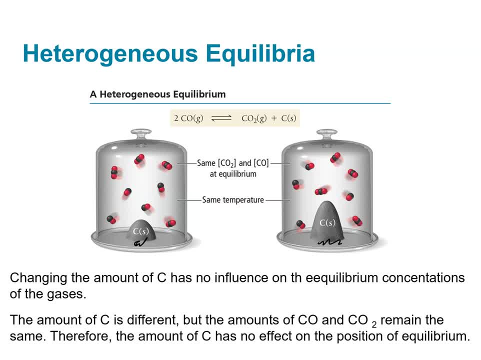 And here we have a much larger pile of Solid carbon. But changing the amount of this Solid carbon has no influence on the equilibrium Concentration of the gases. If we have Double or triple the amount of carbon, Nothing shifts the equilibrium. 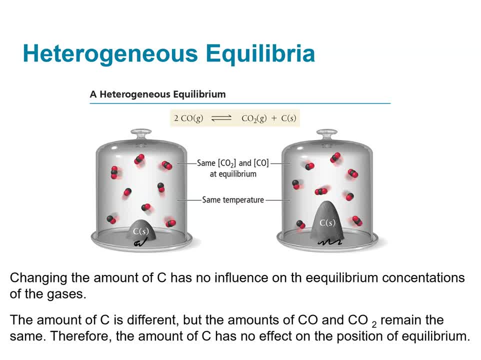 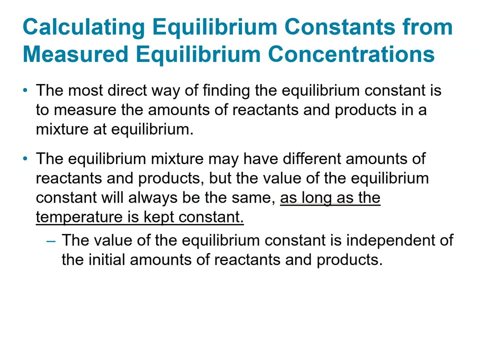 Of the reactant gases Or the product gases. This means it literally does not participate In the equilibrium determination Of reactants and products, So we just exclude it. Kind of a nice little proof of concept. So how do we calculate? 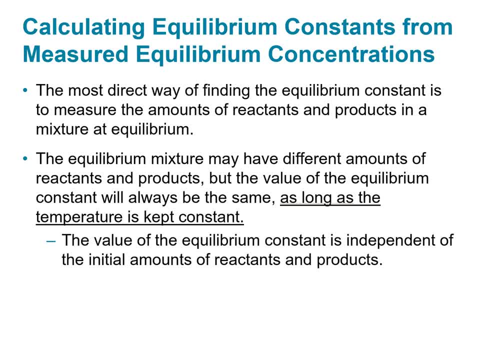 Equilibrium constants From measured equilibrium concentrations. And this is where We're going to start adding some complexity, Because everyone at this point Is probably nodding their head. It's like, okay, I got this, The real trick, Which we're going to spend most of the second lecture on. 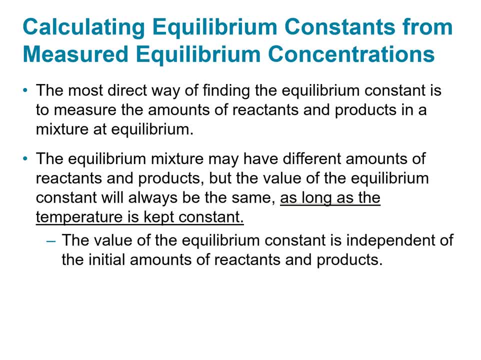 Is: how do we use these relationships To predict things? Because that's what chemistry is all about: Using these chemical models To accurately predict Things in nature. So the most direct way Of finding the equilibrium constant Experimentally Is to measure the amount of a reactant. 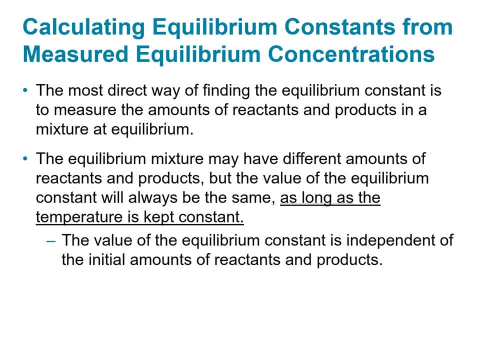 And products in a mixture At equilibrium. That's the most direct way to do it, And then you can plug those right into The equation to determine K. Now it's important to note The equilibrium mixture Might have different amounts Of reactants and products. 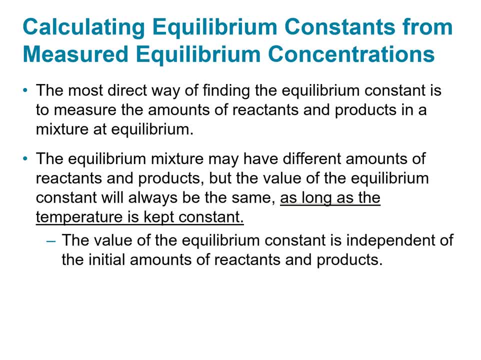 Between different Equilibrium mixtures, But the value Of the equilibrium constant K Is always going to be the same As long as the temperature is held constant, Because you shift equilibrium with temperature And we'll get more into that detail later. 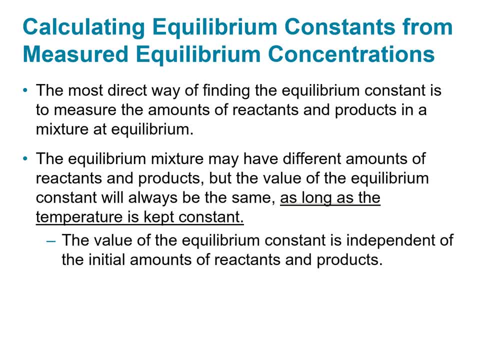 But equilibrium constants Are specific to the temperature Of a reaction. Another way to say this Is that K Is independent Of the initial amounts of reactants and products. So if you set up a reaction, K is going to be K for that reaction. 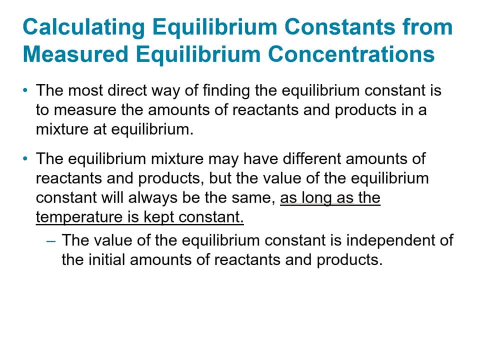 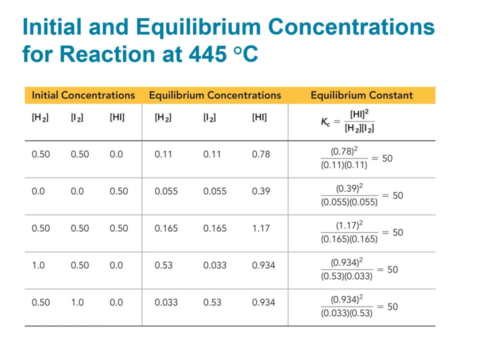 Regardless of how much Reactant and product you have, If you let it reach equilibrium. A good example of this: All these reactions Are done at the same temperature, 445 degrees Celsius, And it's that Reaction we were looking at earlier. 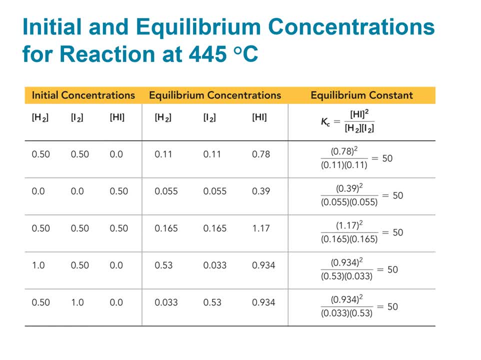 Where we have one equivalent of hydrogen gas Plus one equivalent Of iodine gas, Makes two equivalents of hydrogen iodine gas And that gives us the equilibrium expression We see over here in the top Right corner Of the chart And you can look for this array. 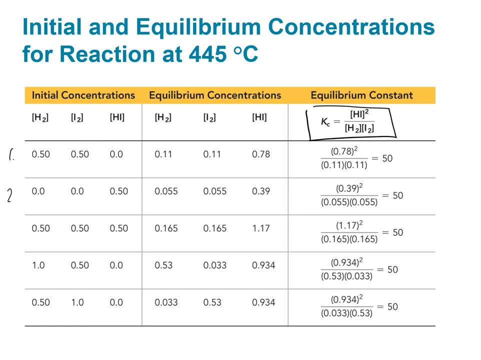 Of different reaction conditions. We have reaction condition one, Two, Three, Four, Five Different sets of reaction conditions. We have different initial concentrations Of hydrogen And iodine Or, in the second condition, It's all hydrogen iodide gas. 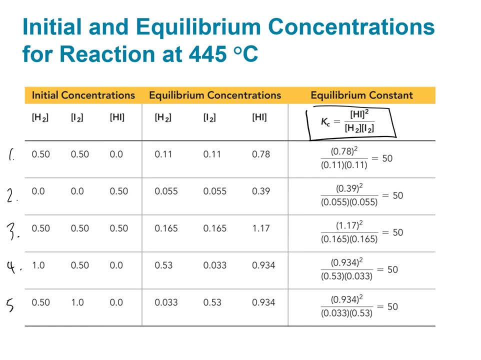 All product Initially, Or we can set up with equal concentrations of each. None of this matters, Because if we let them reach equilibrium And we measure their values at equilibrium, Doesn't matter where we started. It matters where we ended And when we plug those values in. 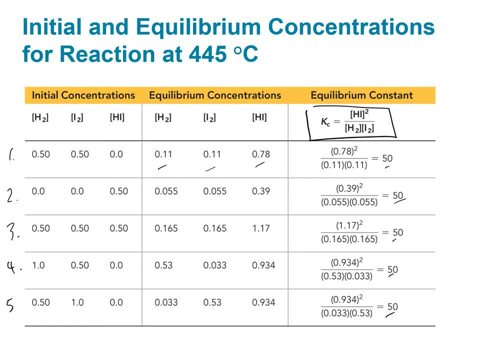 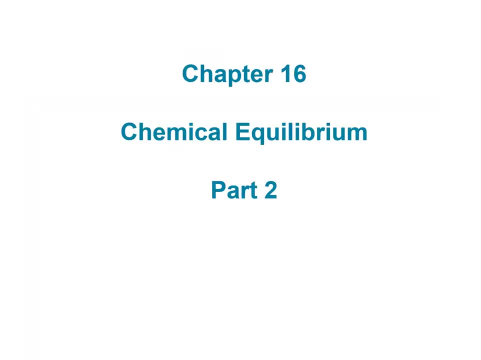 We get the same Value for K 50. Across the board. So this is going to be the end of lecture one And we're going to pick up Lecture two. It's just going to be a click away for you guys. 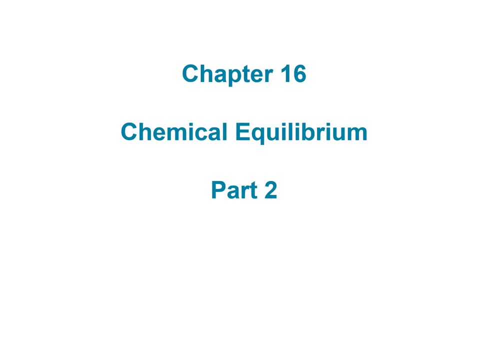 So Join me For the rest of the chapter. If you Take a break, Stretch, Maybe take a day. Part two here, Chapter 16..